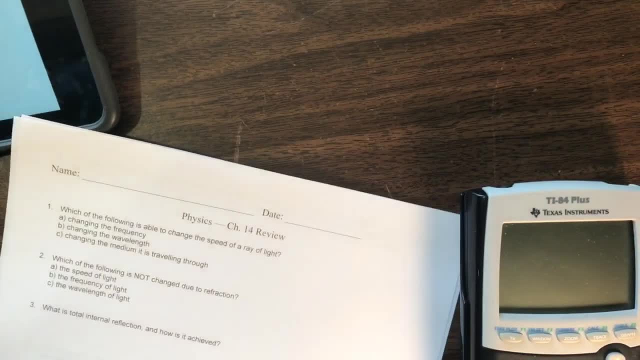 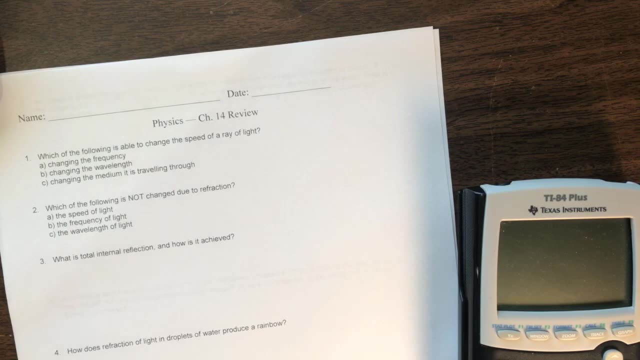 Alright, good afternoon everybody. We are going to be finishing up. what was it? 14C, I think it was- And we are going to, after that, talk a little bit about the test. So let's go ahead and get started. 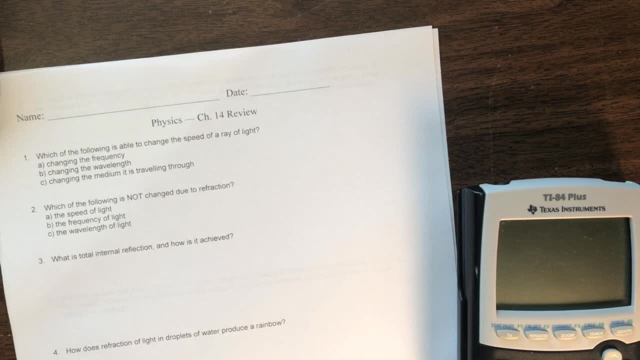 You guys can say hi to me in the comments section and if you guys have any questions at all, go ahead and ask. So today we're going to be looking at first of all, like I said, 14C. Let me see if I can pull it up in the book here. 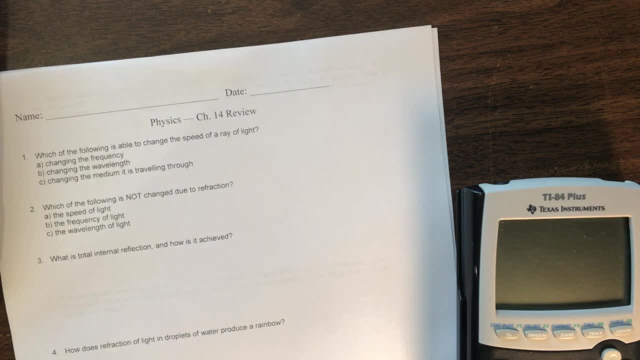 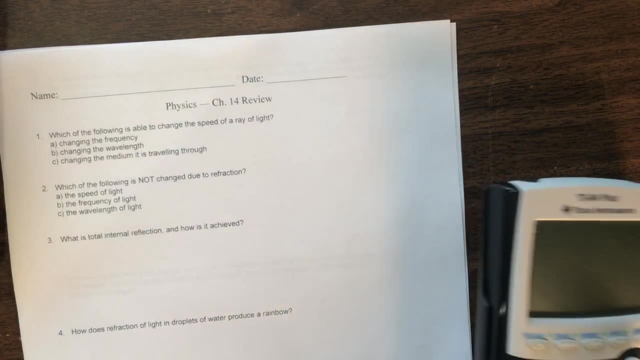 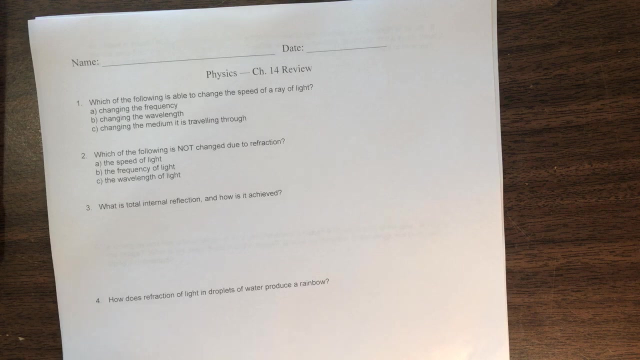 Make sure you check out. I've already posted the review guide for you guys. The test this time is not going to be as long as last time, so we've got only one chapter. and it wasn't a very long chapter, It was only like A, B and C. so we've got refraction, you've got total internal reflection and you've got the lenses. 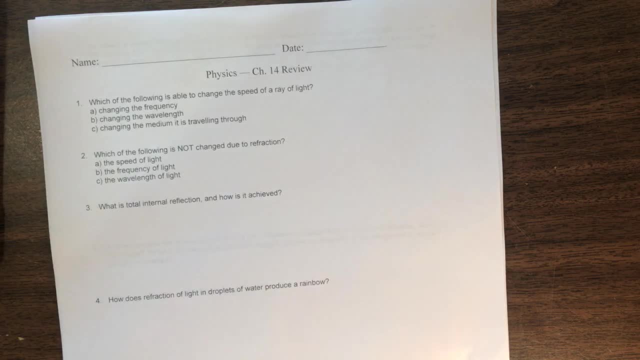 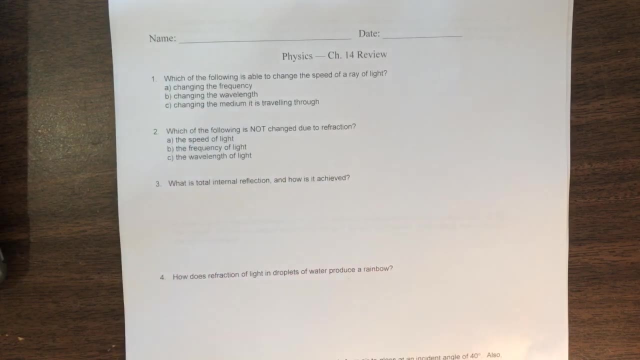 Now you do have two different kinds of lenses, both the converging and diagonal Diverging stuff, so expect to have questions on both of those kinds And so make sure you guys check up on Google Classroom and see that we have the review up on Google Classroom. 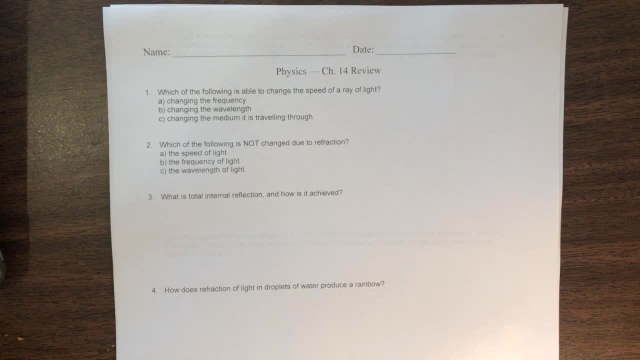 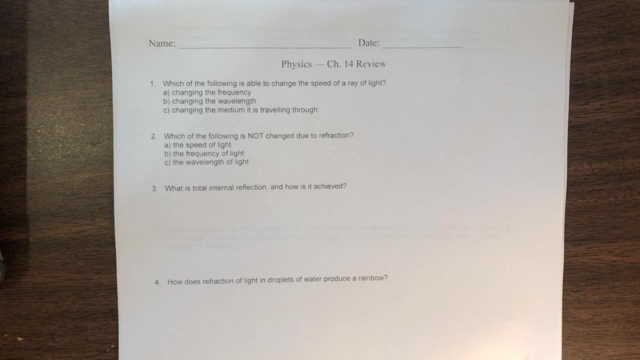 So let me see if I can pull up the homework and we'll go through that All right. So this one was pretty much all about critical angles And let me see we did 14C. just one and four, and I think four had multiple parts to it, right. 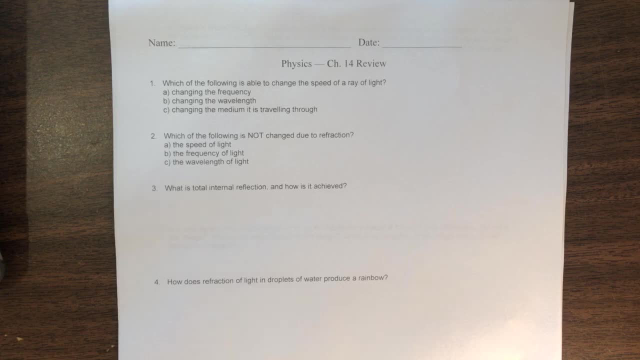 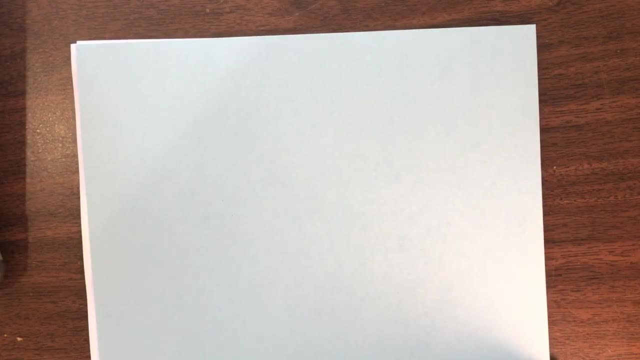 Maybe. Yeah, 14 had multiple parts to it, Okay, So let's go ahead and do that now. All right, So 14, number one: we have glycerin, which is used to make soap and other personal care products. Glycerin is actually a natural component of natural soap, or I mean, I don't know if it's natural soap, if that's the way you'd call it, but the original soap. basically, if you take fat and react it with sodium hydroxide or lye. 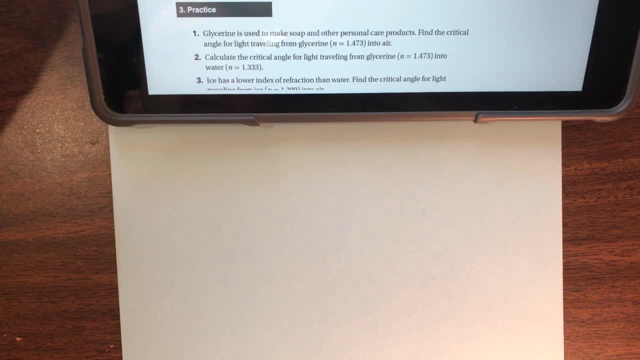 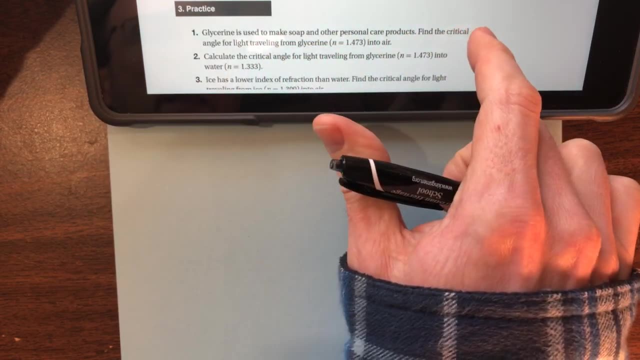 which is known as soap. sodium hydroxide is known as lye. you'll get out your fatty acids, salts, which is soap, and glycerin. okay, Glycerin is a natural moisturizer. All right, So it's used to make soap and other personal care products. 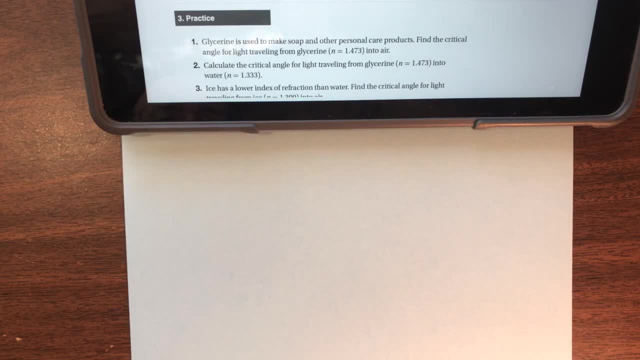 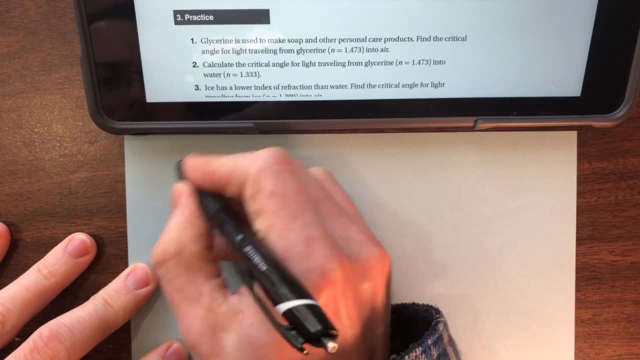 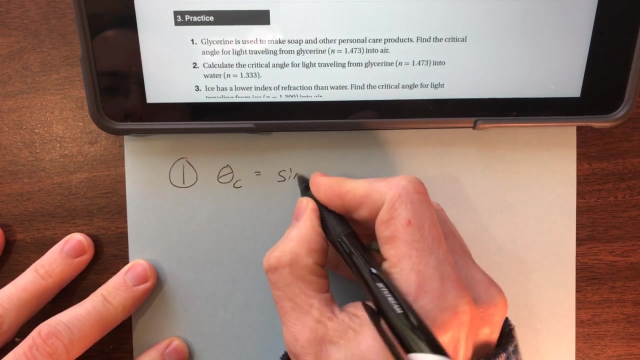 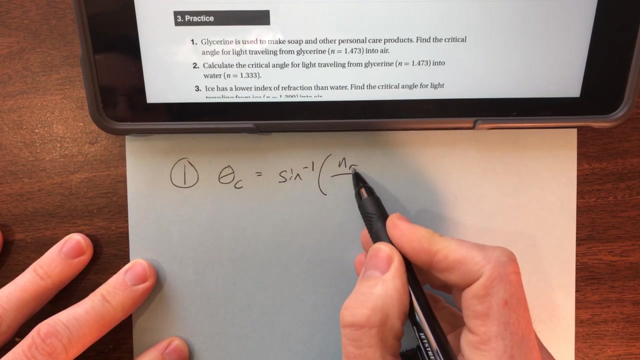 find the critical angle for light traveling from glycerin into air, And so we can go ahead and do that. Your equation, if you recall, was simply: the critical angle equals the inverse sign of your index refraction of the material that has the refraction in it. 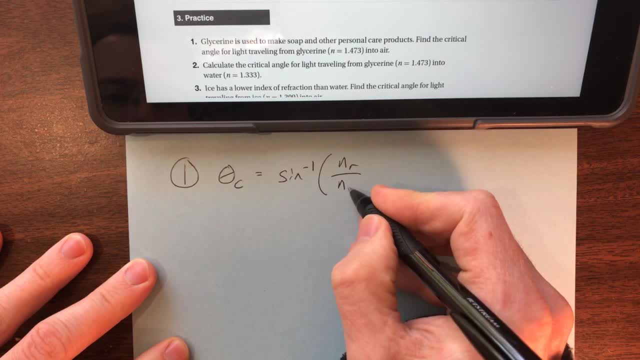 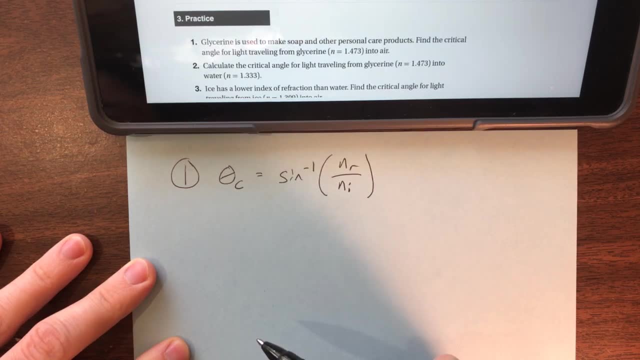 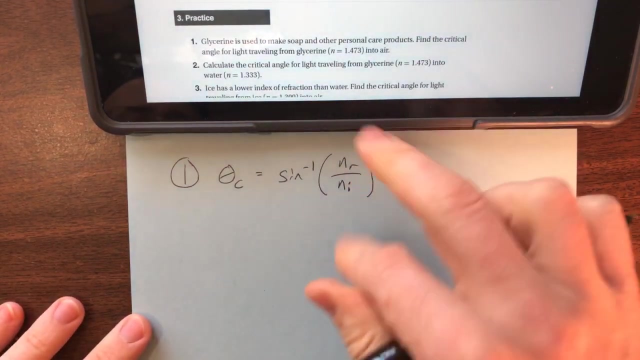 and the index of refraction of the incident material, so where the light's coming from and where it's going into, okay, And so one of the biggest mistakes that you could possibly make on these kinds of problems is just switching an R and an I. 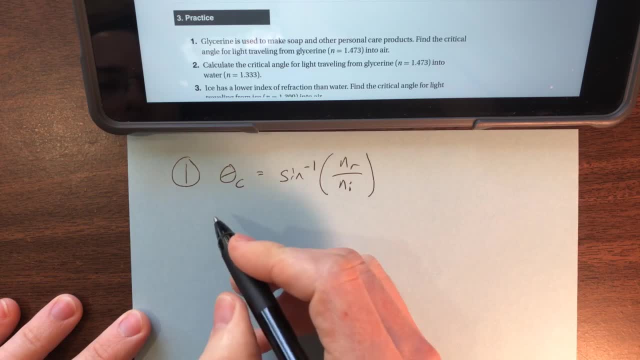 and so that's an easy, easy mistake to make, so make sure you don't do that. All right. So, number one: we have glycerin. It's used to make soap and we said we're going to find the critical angle. 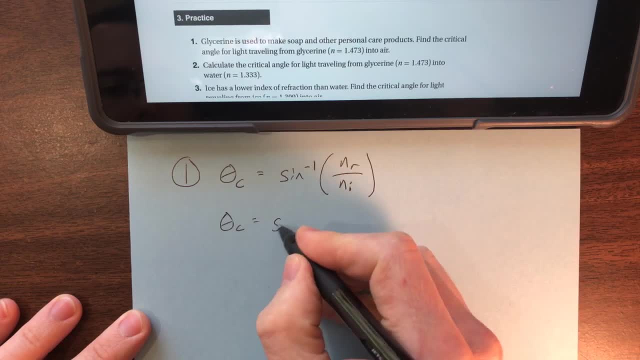 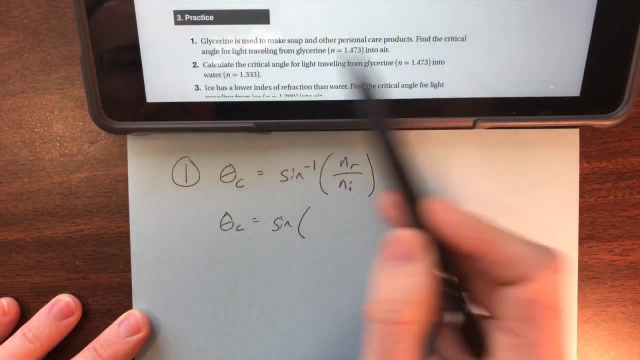 so we're just going to plug it in. Here's the critical angle. It's going to be the inverse sign of now which one goes on top. It's going from, it's traveling from glycerin. so that's the incident material. 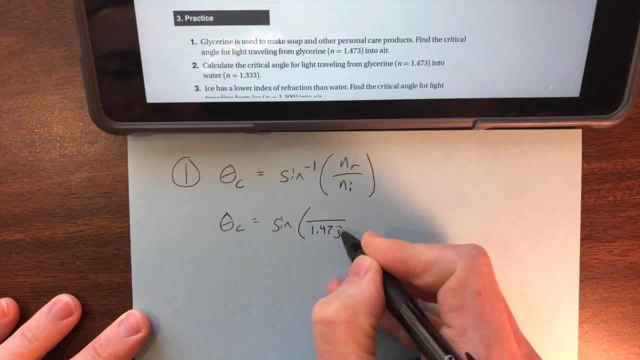 so we're going to put our 1.473 here on the bottom and on the top it's going into air. one Notice: if we switch those, you wouldn't be able to get in, You wouldn't get any kind of answer. so this is the inverse sign. 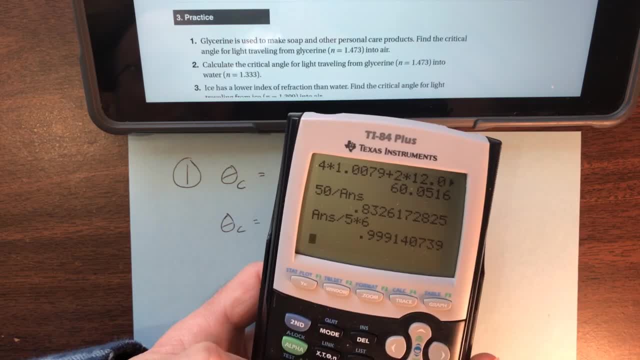 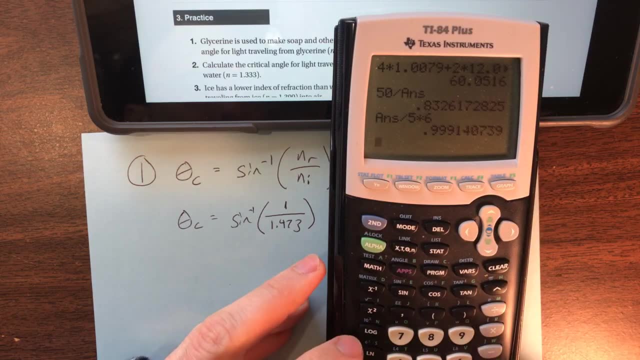 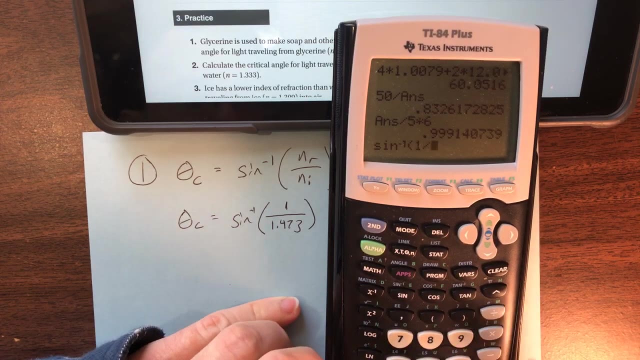 Let's even do that right now. So make sure that your mode is set for degree mode, right? And let's go ahead and plug this in. So if we have the inverse sign, so second sign, you're going to get inverse sign of 1 over 1.473,. 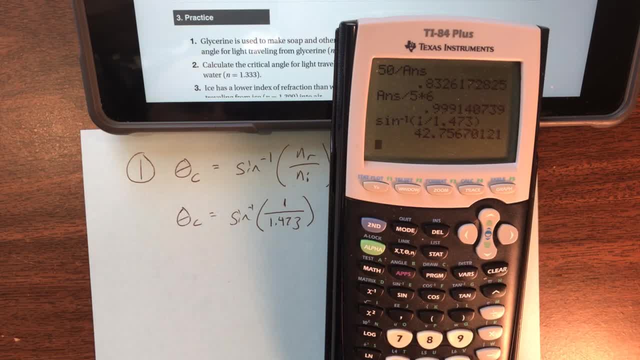 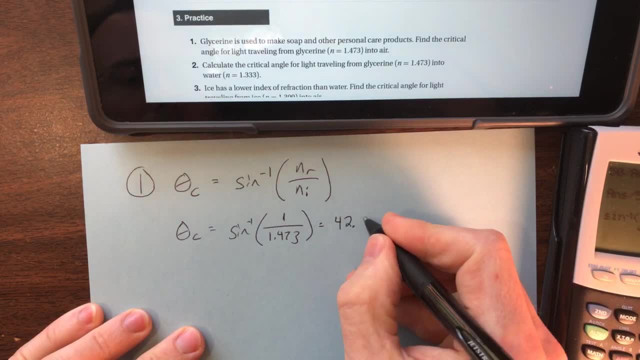 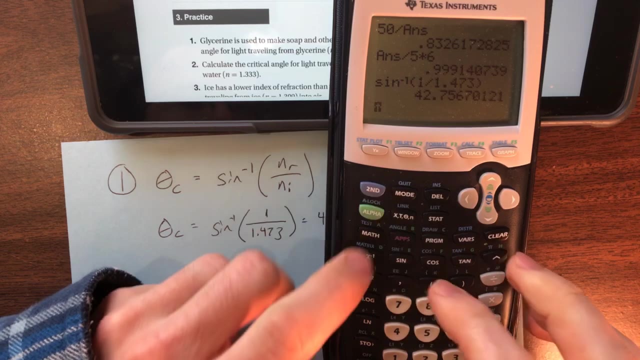 and we get out 42 point. well, round it up to 42.8 degrees. Forty-two point eight degrees. Now notice, let's just for fun see what happens if we switch them right. Let me just show you, guys. 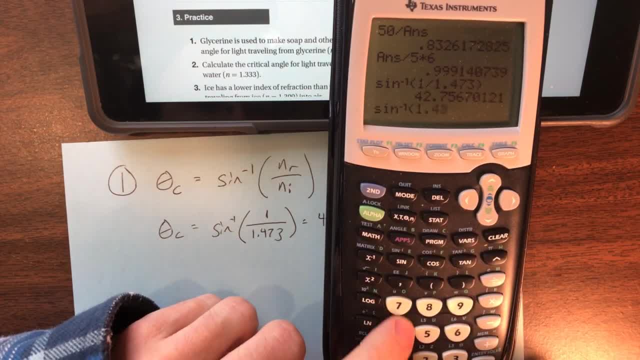 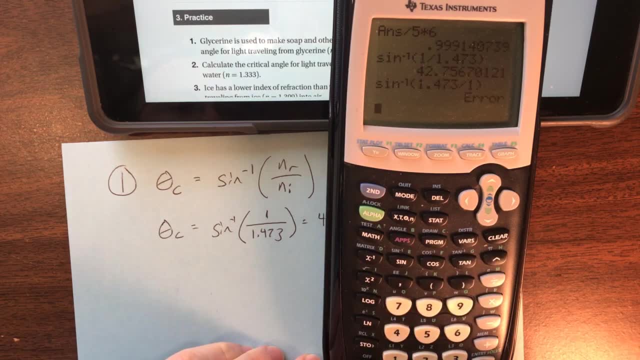 So if you switch them and put 1.473 divided by 1,, what you're going to get is an error. And well, why do we get an error? Because the sign of something can never be more than 1, right? 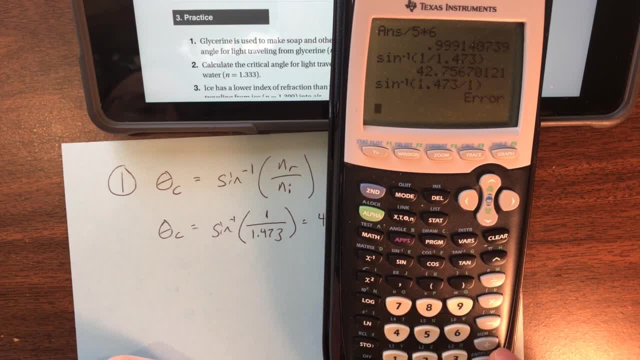 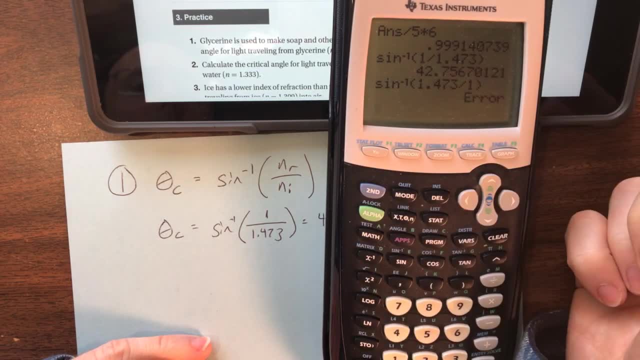 The maximum you can get is 1.. Or, yes, You know, it's between negative 1 and 1, inclusive, right, And so this is saying: okay, you get an inverse sign of something that's larger than 1,. 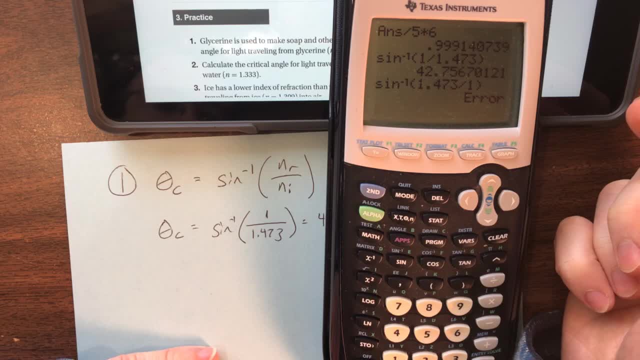 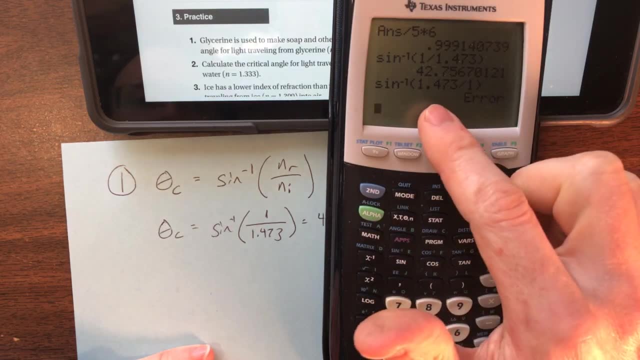 then that's impossible. It's impossible to have the inverse sign of something larger than 1.. And what would that mean? If you had something where you would have, you'd try to calculate the critical angle for something that was like this, where the bigger number's on top and the smaller number's on the bottom. 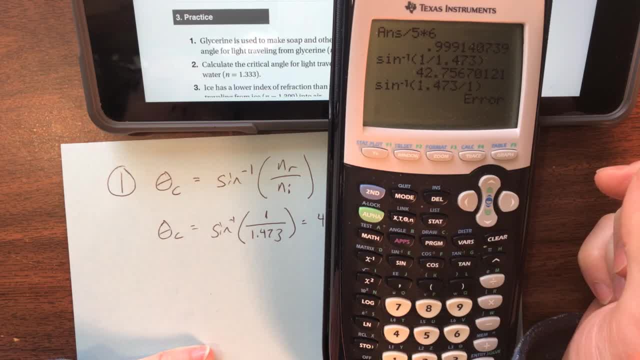 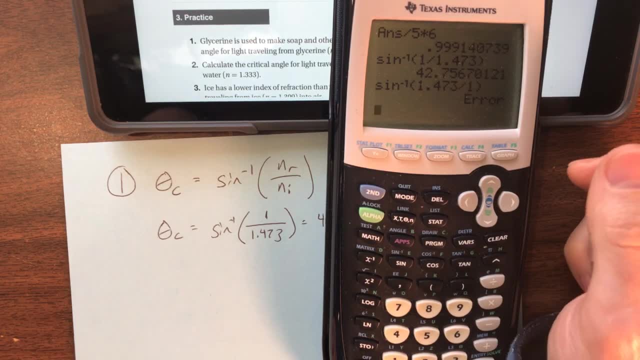 you would simply just have no critical angle. There would be no angle at which all of the light was internally reflected. So no possible angle. all right, That's what would be the case. Okay, So that's number 1.. 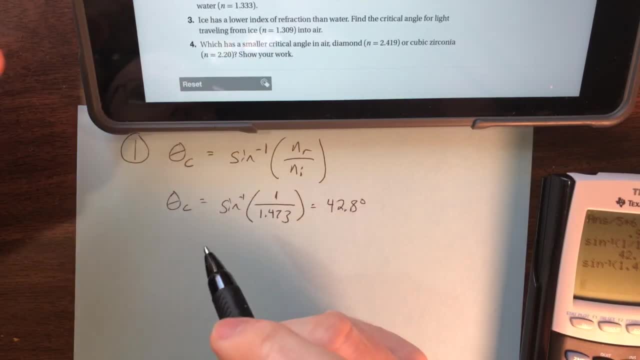 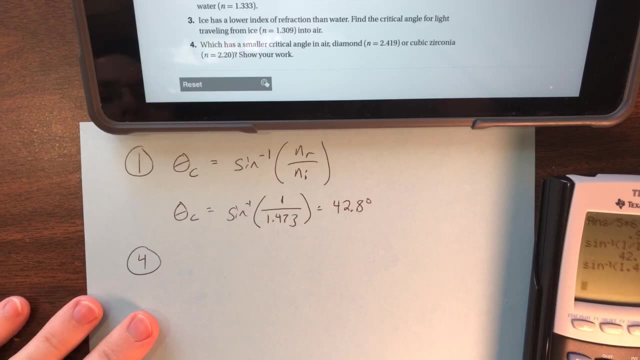 Number 4, going down here to number 4,, which has a smaller critical angle, Let's just go ahead and solve for both of them. I wouldn't so, as I show your work, so you don't want to just guess on this one. all right, 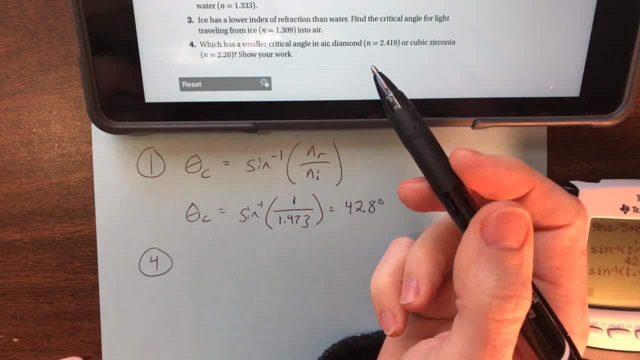 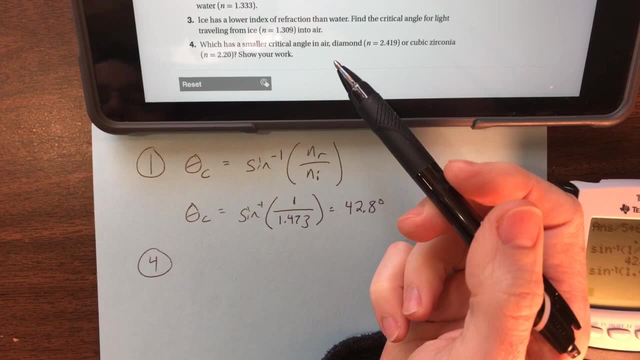 So, but we can, you know, make a guess ahead of time and say, okay, well, it would make sense for diamond right to have the smallest critical angle here, because you know it's diamond, it's the expensive material, plus diamond has a larger index or a fraction. 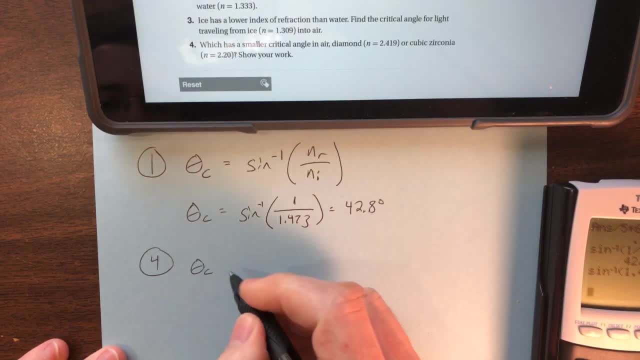 But let's actually go ahead and calculate these things, okay. So you have a critical angle, for let's do what do you want to do first. Let's do the qubit zirconia. Let's just we'll call that qubit CZ, okay? 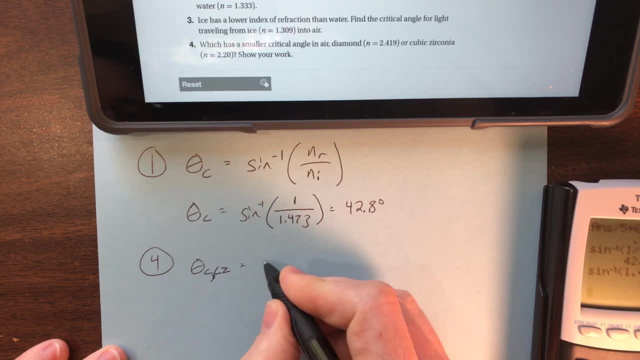 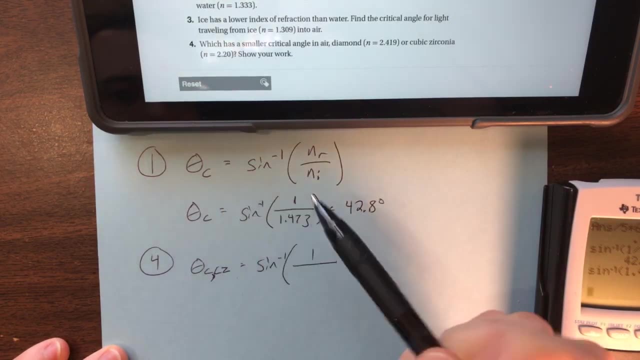 So this is the critical angle of, And so this is going to be the inverse sine of 1 over what That's, 2.2, right, And we're always going to be putting here, in this case, the value for air on top right. 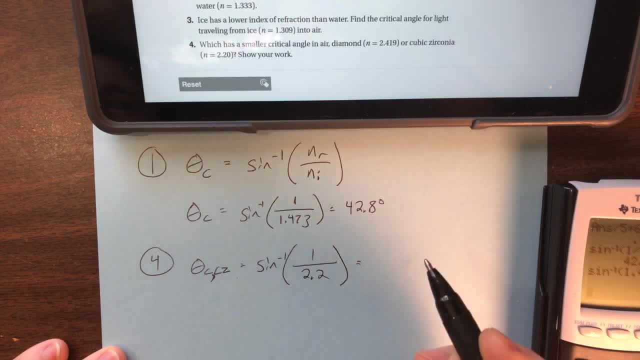 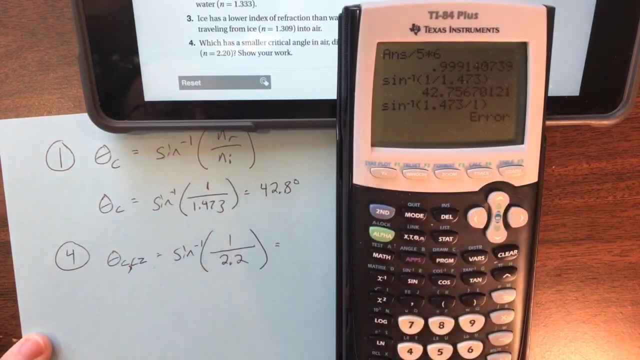 So 1 on top. Obviously, if the gemstones were in some other material, like water or oil, this number all of a sudden would change, right? But now it's just asking smaller critical air. Well, it says right here in air. so we're just going to put 1 here on top, all right. 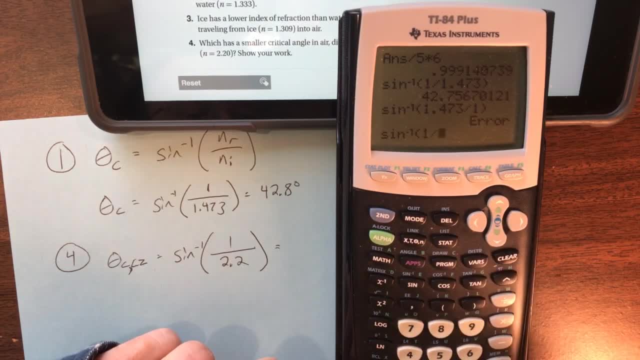 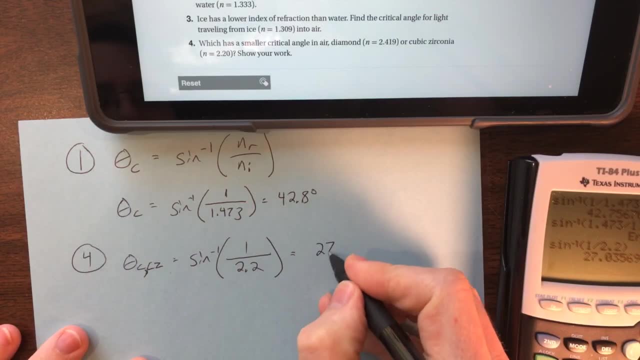 So this is going to be 1 over 2.2, which is 27.. That's pretty small. That means all angles greater than 27 degrees are going to be totally internally reflected, which is pretty significant. So that's all the angles, unless, so it pretty much has to come at- 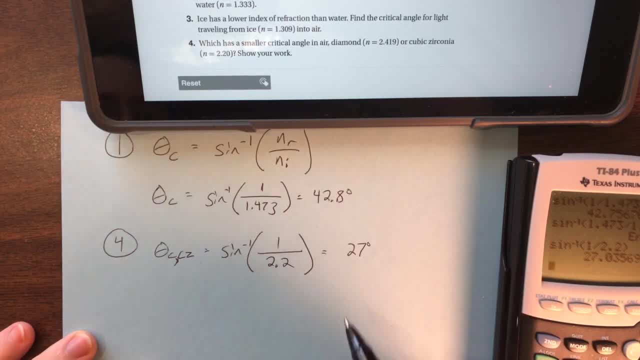 you know, close to perpendicular right, And if it's not, it's going to be internally reflected. And so what happens is for these gemstones, when the light comes in, is actually internally reflected quite a bit until it hits like one specific face or hits at the face. 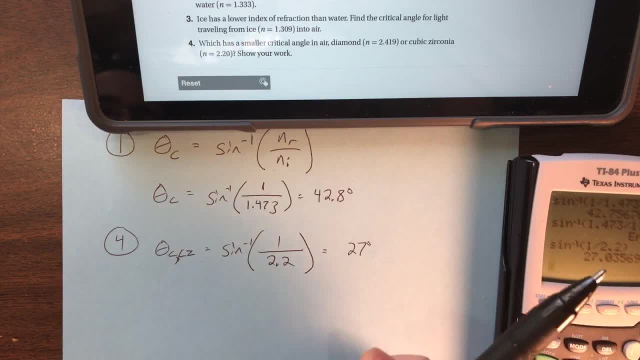 in a certain way, the light comes straight out, And so that's how they're sparkly. So most of the light stays in, but then more like it's concentrated at the certain points at which, like the Okay light's going to come out and sparkle and you'll notice it there. so it's essentially taking some 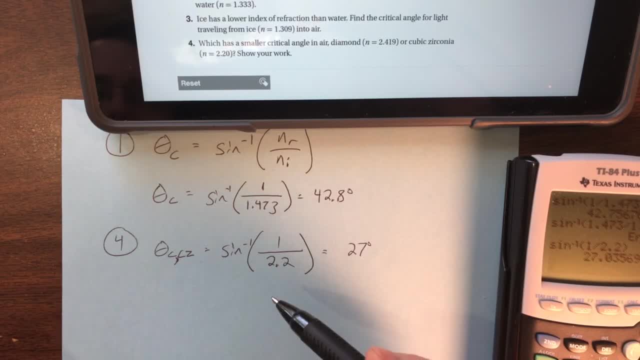 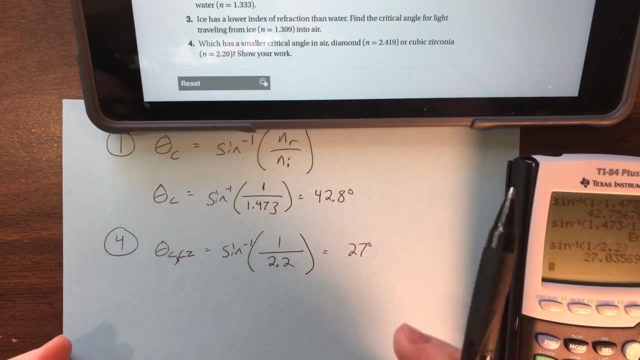 of the light. so the light's not going to be able to stay inside a gemstone. it's eventually going to come out after bouncing around a lot, and that's where the cut comes into play. right, you want to cut the gemstone specifically such that you can get the light to come out at certain spots, and 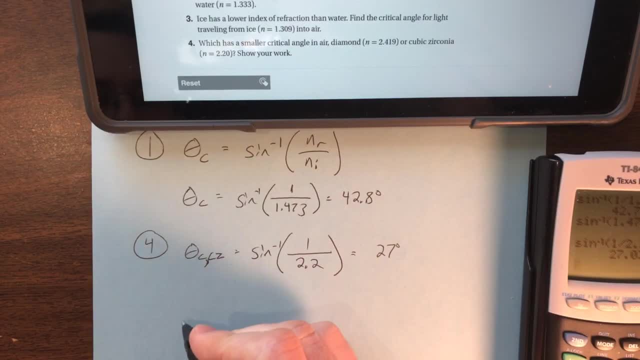 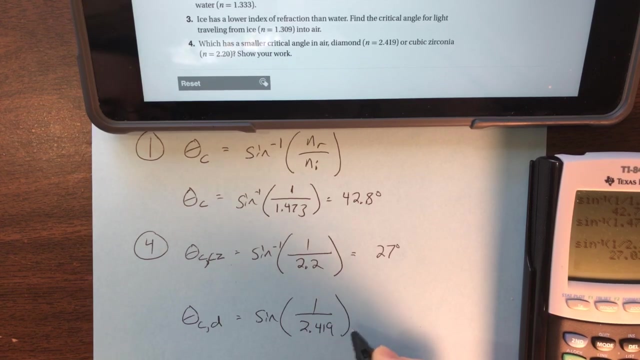 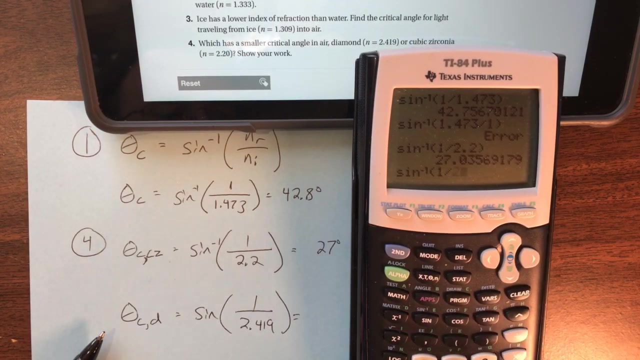 make it look like it's sparkling, right. so that's that's done on purpose. all right. so we have the critical angle once again for diamond gonna be the inverse sine of one over 2.419. let's get that inverse sine of 1 over 2.419 and that gets us 24.4. 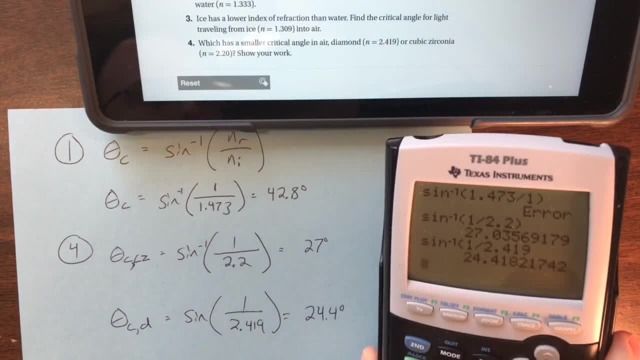 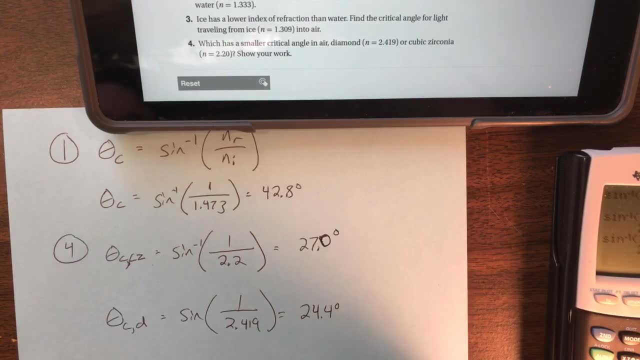 24.4 degrees. what was the other one? that was 20, 27.0. okay, so we'll just put that in 27.0 degrees, all right, and so we just say okay. the question is, which has the smaller critical angle? well, this one right, 24.4 is smaller than 27.0, so this is smaller. 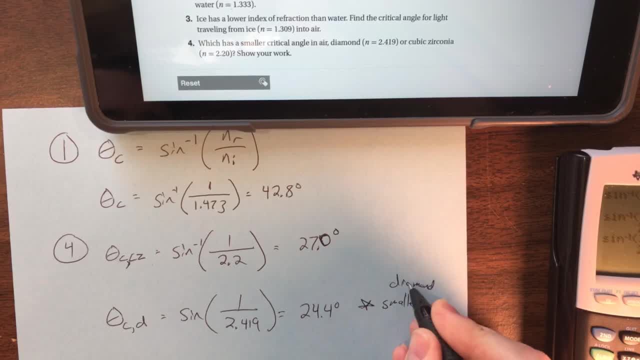 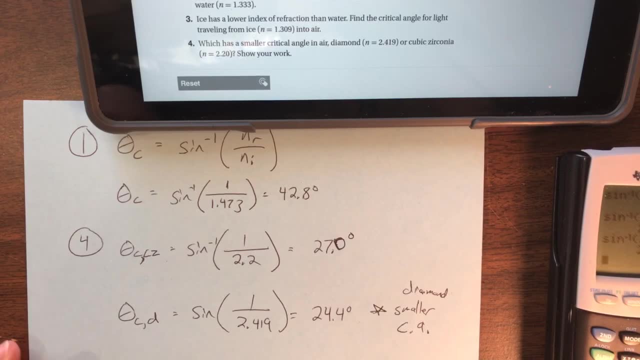 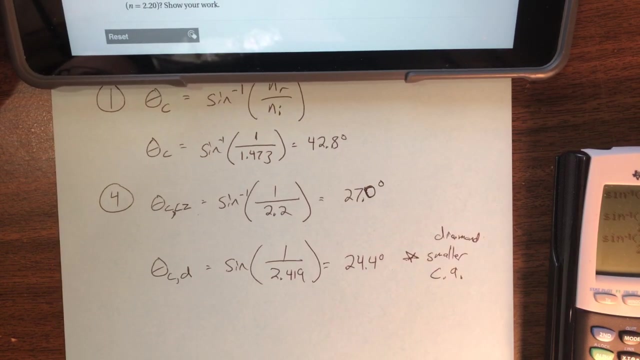 so we say diamond has the smaller critical angle. all right, and that makes sense. it goes along with our prediction prediction because it's more expensive, because it's got the higher index of refraction and, by the way, there's actually a gemstone that does have a higher critical. um, well, it has a higher index. 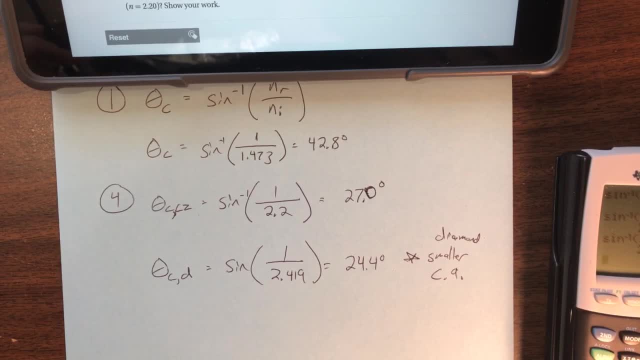 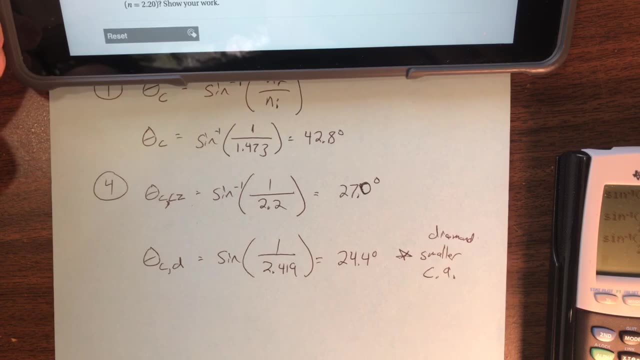 refraction and a smaller critical angle. i forget what it's called though, um, but it's. it's actually got a larger index refraction than diamond. pretty cool, but it's actually cheaper. but so it's not necessarily just, you know, the more expensive one that is better, but most of the time diamond is. 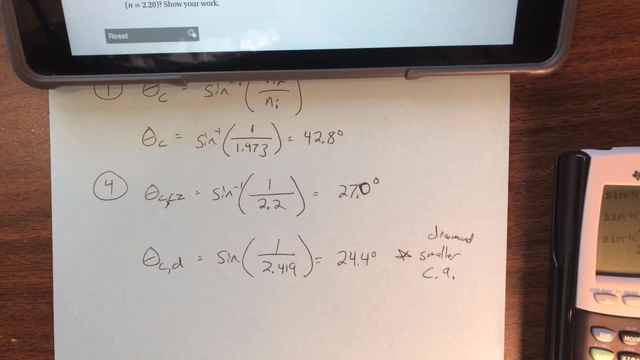 pretty awesome and it's going to beat other gemstones in a lot of different ways. so, anyway, that's pretty much it all right, we have a test coming up, so no need to rush it. i hope you guys did manage to watch those videos. like i said, we we can't really do a lab and i think there's no point. 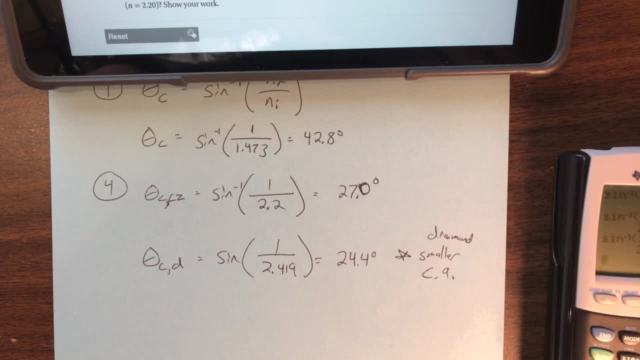 in us actually going through having you guys do all those calculations with those videos, because they're the same kind of calculations that we've done and the whole point in doing a lab is so you can do the hands-on work right, and if you're not doing the hands-on work, i'll just let you guys. 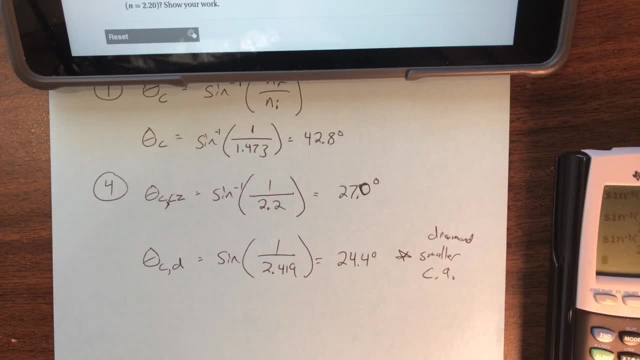 watch the videos and we're good, so please, guys, do watch the videos. there are two demo videos about this kind of index refraction and those um refraction, all that kind of stuff, so make sure you watch those videos. yeah, snell's law. and the other one was something um some guy messing around with corn oil and broken glass, so be sure. 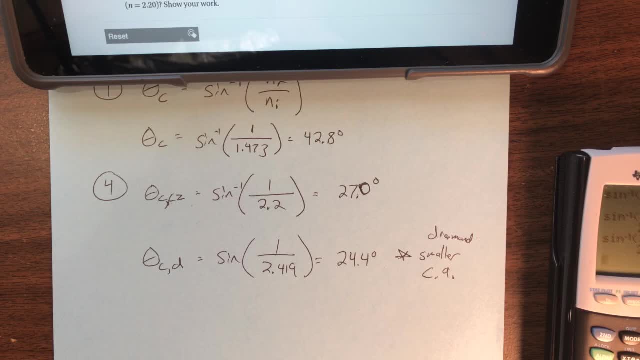 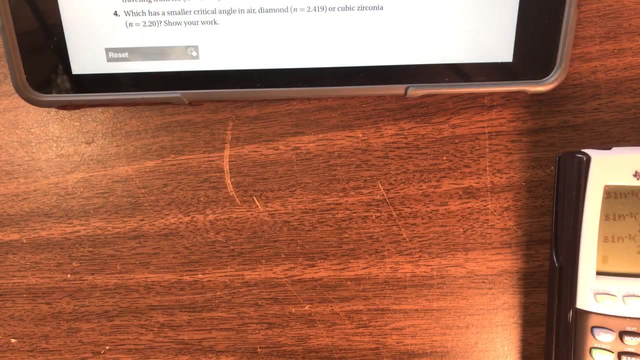 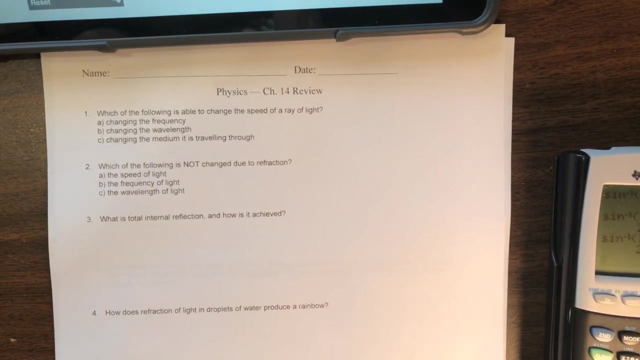 to check those out. they're actually pretty cool, but, um, yeah, that's it. you just watch them and that's it. now we have, like i said, a test coming up. you guys got plenty of time to review for this, this homework. however, i'm going to make this do on friday, and so we'll go over the answers on friday, so please treat this. 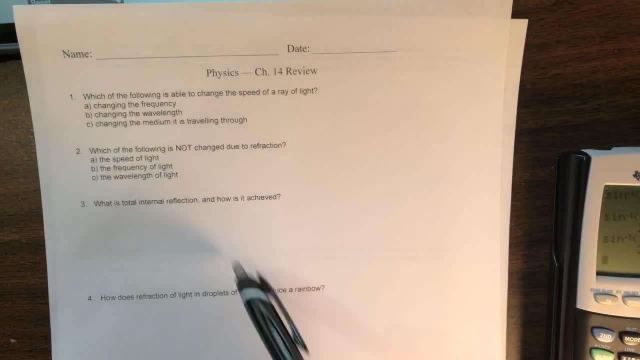 as a homework. you are going to get a grade for it, so treat as a homework, do this, and it's also going to serve as your review. all right, so go through these problems. it's up on google classroom- and then we'll talk about the answers on friday and your test is going to be on monday, so that's it. 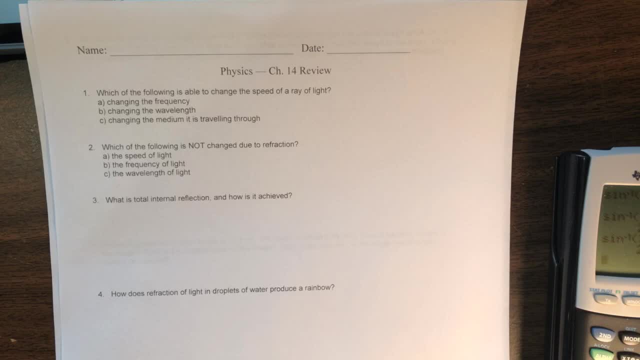 you guys have any questions, anything at all, hannah adam, anything at all and uh, nope, okay, good, i thought this section wasn't too bad, so hopefully you guys make some sense of it and test on monday. so let's, let's all do really really well on this test. so i know it's open notes, but that doesn't. 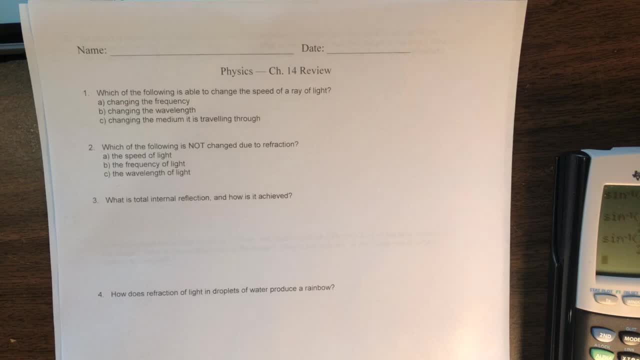 mean you guys can't make mistakes, so please try to make sure you have the correct units on things. double check your answers and get this stuff right. this is a test i think you guys can all do. well, we've done the the ray diagrams for mirrors, so you guys can do the ray diagrams for lenses and um. so 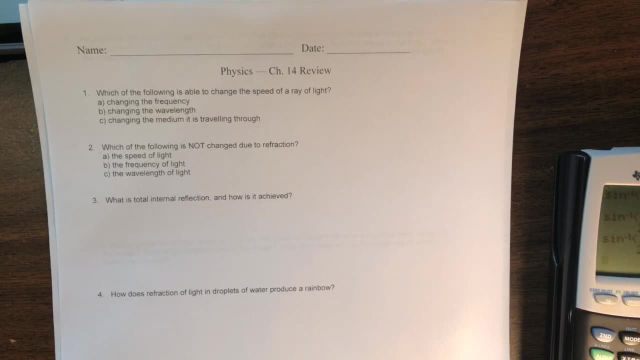 yeah, so good luck. we'll talk on monday, so just this is homework. yeah, this is the only homework, that's it. um, how's the chess tournament? the chess tournament's going all right. um, adam, have you won your bracket? i was expecting you're probably winning your bracket. i am, i believe, leading in my bracket. i've won two games and 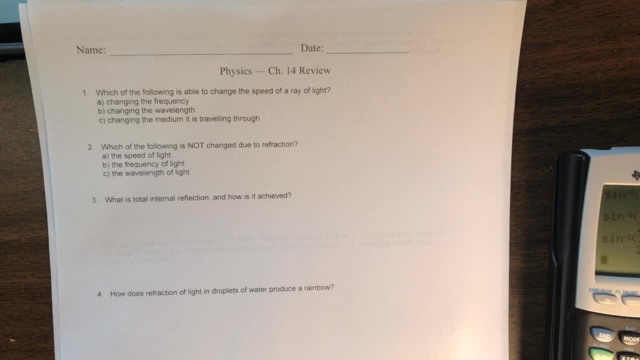 i got a couple games left just going. you know it takes a little bit of time. you did win awesome, all right. and then we have- i don't know about the middle bracket- who won in that one, and all that kind of stuff. we'll, we'll see. 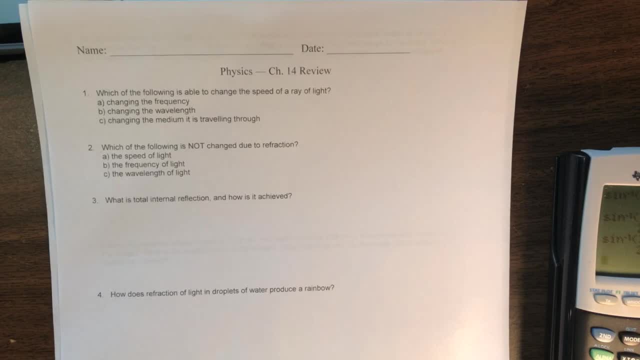 so, and then it's, i think, as soon as the first um you know three, like the all, everybody's all done their initial games, then our, our final three, will be playing. so adam is in the final three and we'll see how that goes. cool, so yeah, once again, please do.